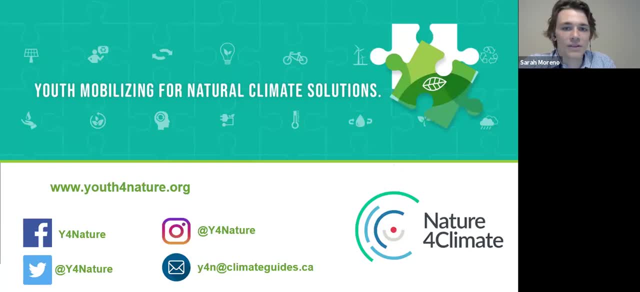 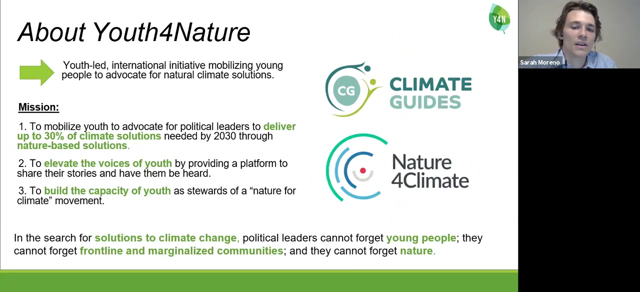 So what is Youth for Nature? It is a youth-led international initiative that is mobilizing young people to advocate for nature-based solutions or natural climate solutions. It's supported by Nature for Climate, an international organization of NGOs and international organizations, including the Nature Conservancy the UNEP. 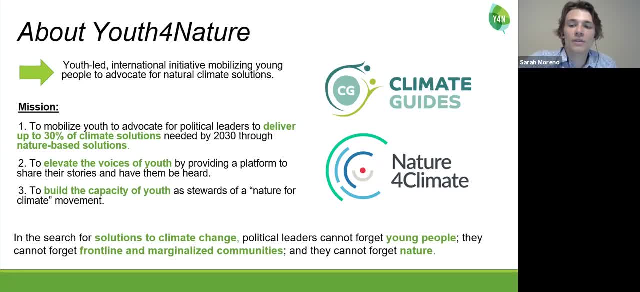 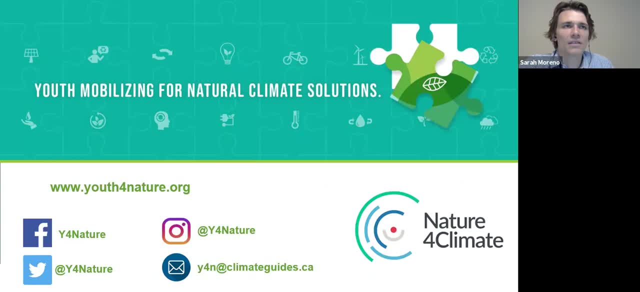 and Conservation International. It's advocating for natural climate solutions to be included in the climate plans of countries. So you might be willing to ask: why natural and climate? Basically because these crises are very linked. We face these two crises at once: the ecological and. 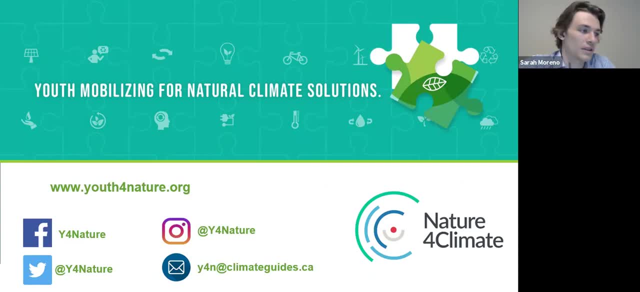 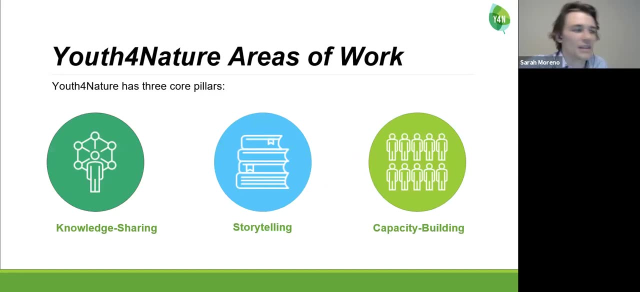 climate breakdown. We cannot address one without the others. So what do we do? Youth for Nature is acting in three ways. We advocate and share knowledge on natural climate solutions. We try to elevate the voice of the youth by providing them a platform to share their 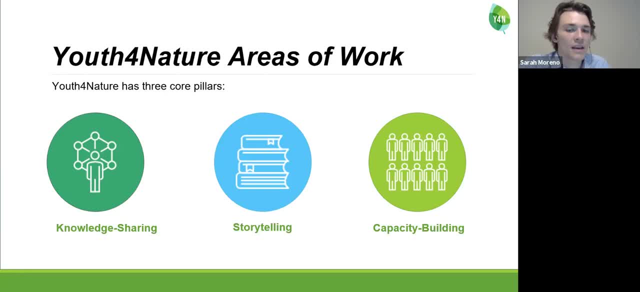 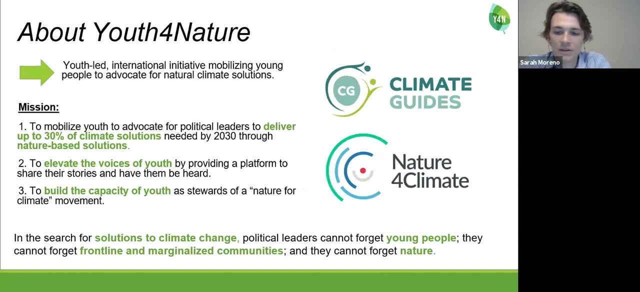 stories and have them be heard in the highest instances. And we also build the capacity of youth as stewards in the climate movement. So a word about our missions. past is to mobilize the youth to advocate for political leaders to deliver up to 30% of climate solutions needed by 2030 through 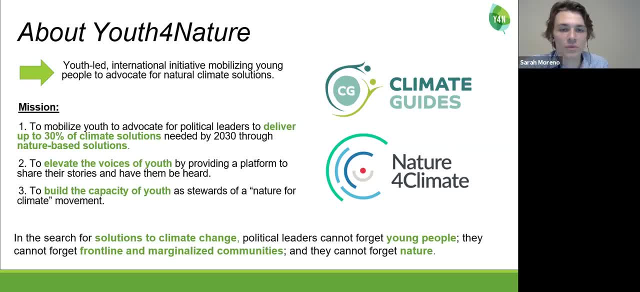 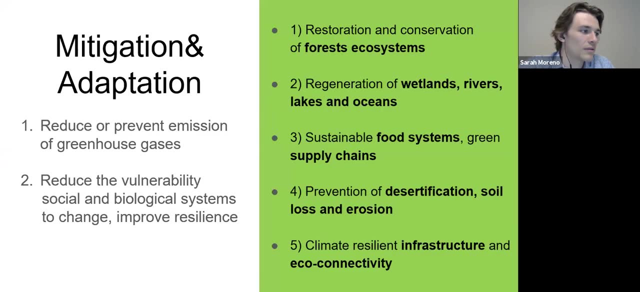 nature-based solutions. Another mission that we have close to our heart is to elevate the voice of youth by providing them a platform to share their story, And we also build their capacity. So I will now proceed to the, let's say, more education part of the 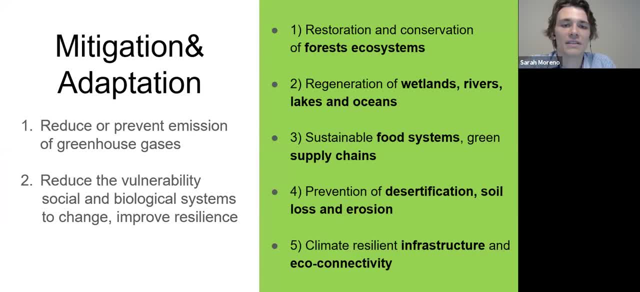 webinar, and then we also have a more awareness and advocacy part. So a little reminder about mitigation and adaptations. I add that the title of the of the webinar was related to it, So the former is the reduction of the factors that lead to climate change, And the later 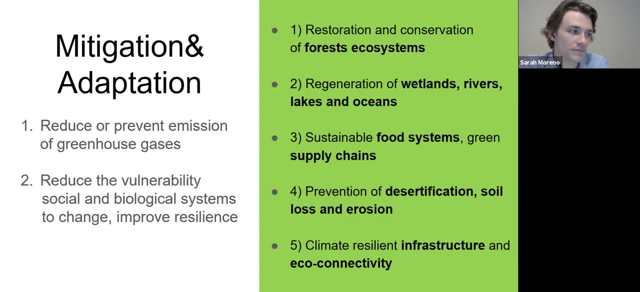 is the reduction of our vulnerability to its impacts. so on the right, you will find listed some types of nature-based solutions- uh, you can read their restoration of conservation of forest ecosystems. also important are wetlands, lakes and oceans, food systems, the prevention of desertification, soil loss and erosion, and eco-connectivity. so what are exactly? 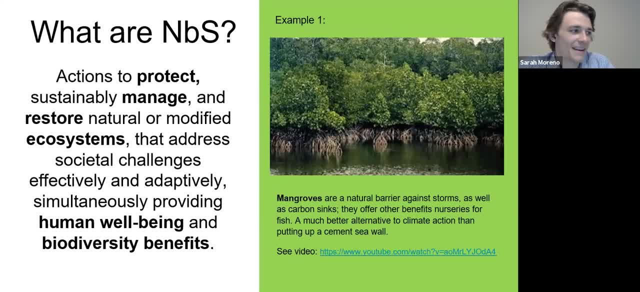 nature-based solutions that i mentioned so many times already. they are action to protect, sustainably manage and restore natural or modified ecosystem that address societal challenge effectively and adaptively, simultaneously providing human well-being and biodiversity benefits. so if we want to make an analogy, we can understand that nature-based solutions. 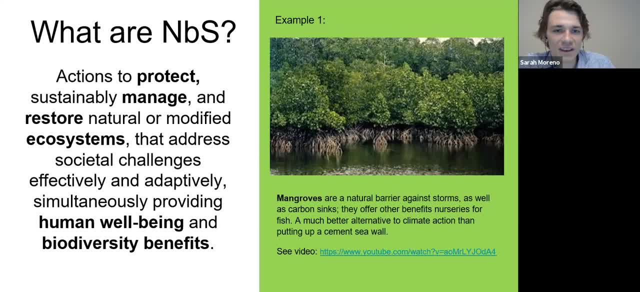 are, as opposed to technology-based solutions, solutions which have been there on this planet, let's say provided by the planet, for centuries and and thousands of years, and which have been proven, which have been, let's say, the the best technology, the best evolutive technology, that 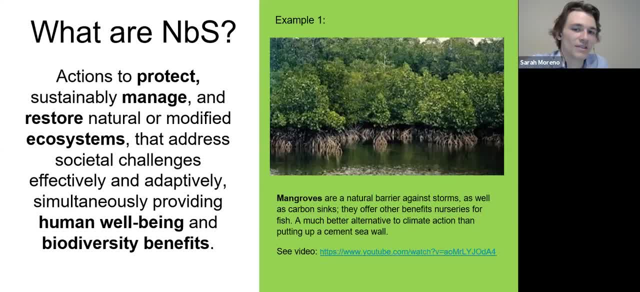 the planet has provided us with. so an example is the conservation and restoration of mangrove forest. mangroves are a natural barrier against storms as well as a carbon sink, so they they suck carbon and they use their grows to stop the rise of the climate change, to the extent that the climate 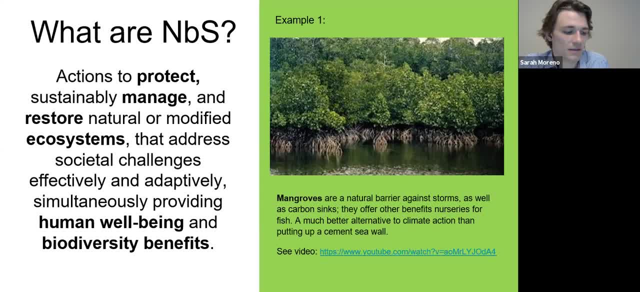 changes are more aggressive or eerie, or uh, they produce a significant amount of greenhouse gas, which uh which increase the climate change, which which increase the effect of climate change, uh. so they offer benny other benefits: co-benefits, biodiversity benefits such as nurseries for fish. 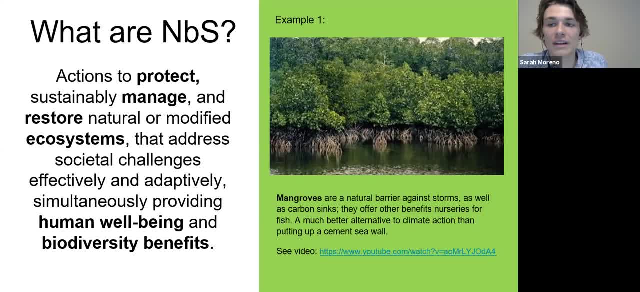 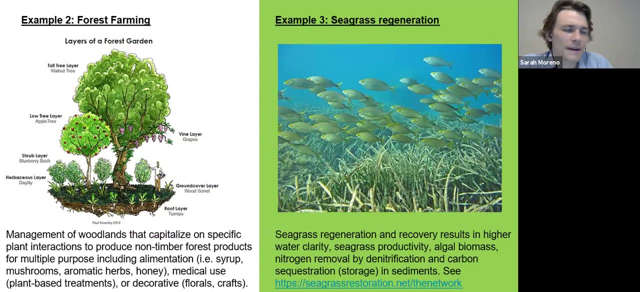 many of the of the ones which are necessary for So. for example, the mangroves are a much better alternative to climate action than putting up cement walls to protect from water rising sea level rise. Other two examples of nature-based solutions are forest farming, which basically also suck. 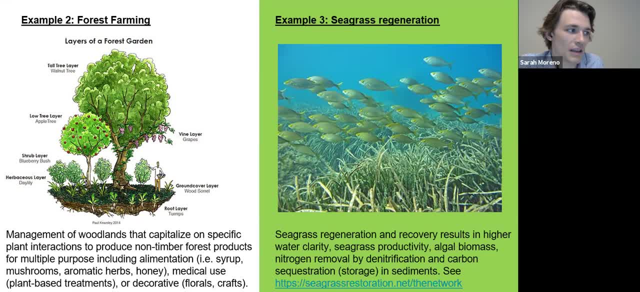 the carbon out of the atmosphere by stocking it in the plants- and not only the trees, but also the plants- And forest farming, as opposed to monoculture, is an example of natural management from which many co-benefits can be derived. 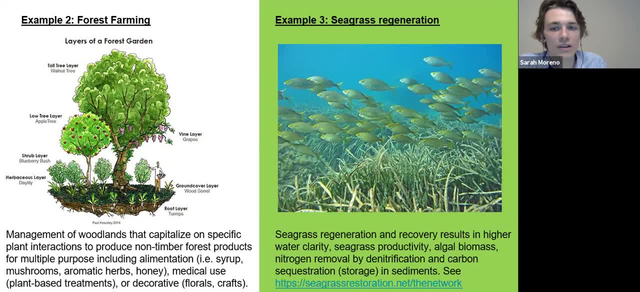 So, additional to lowering the temperature on the micro scale and sucking the carbon, as I said, an appropriate management of forest can also allow to capitalize on soil, So in specific plant interaction, and give co-benefits like other plants that can be. 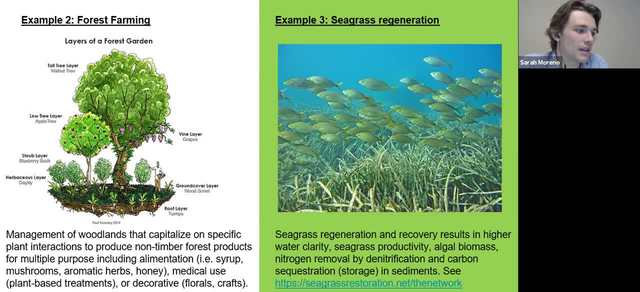 used without cutting the forest. A third example that I think was quite relevant and is not necessarily spoken a lot about is seagrass regeneration. So we were speaking about the restoration of ecosystem. This is a perfect example. So the seagrass regeneration is allowing the recovery of water clarity. 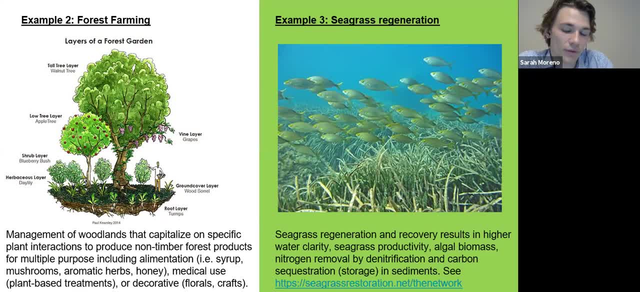 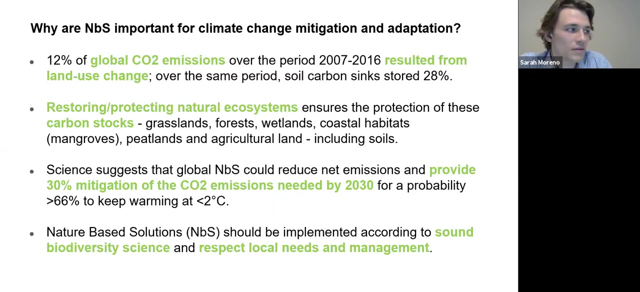 The recovery of ecosystems for living beings, for the fish, for other marine life, and it includes water clarity, seagrass productivity and also carbon sequestration by growing. So I would like to share with you why I think nature-based solutions are important for climate. 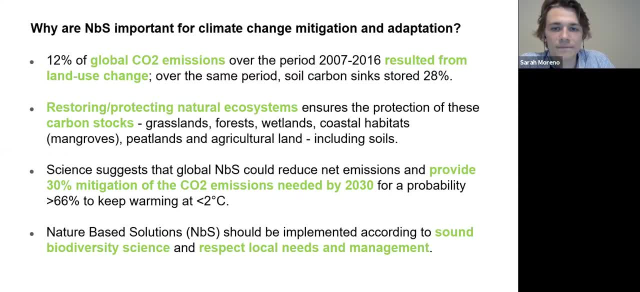 change, mitigation and adaptation. Basically, some of the scientific research that I have put here in the slides show that 12% of global CO2 emissions over the period from 2007 to 2016 resulted from land use change And, over the same period, the soil carbon sinks. 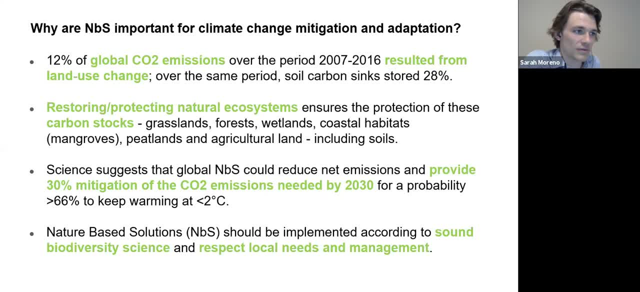 So the extraction of carbon from the atmosphere into the plants or the soil was 28%. It has been proven by scientific research that restoring and protecting natural ecosystem ensured the protection and the formation of carbon stocks and some of the ecosystems I have cited before. So science suggests that global natural-based solution could reduce net emission. 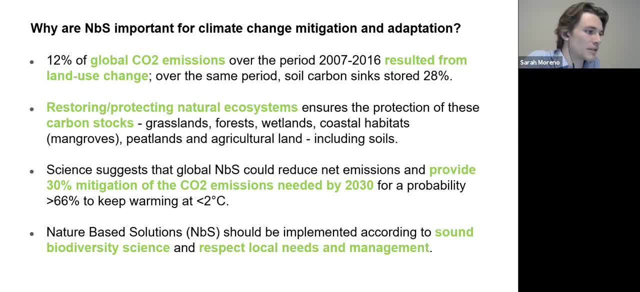 And provide up to 30% mitigation of the CO2 emissions needed by 2030, for a probability of 66%, to keep global warming at maximum 2 degree temperature. And finally, let's say that nature-based solutions should be implemented according to biodiversity. 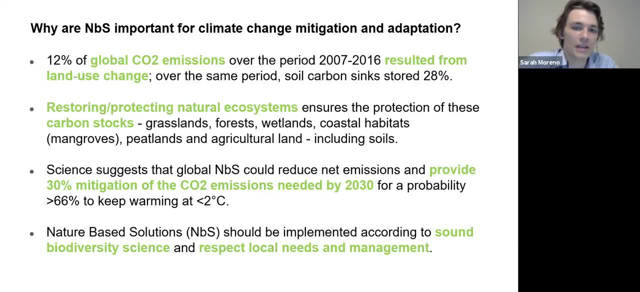 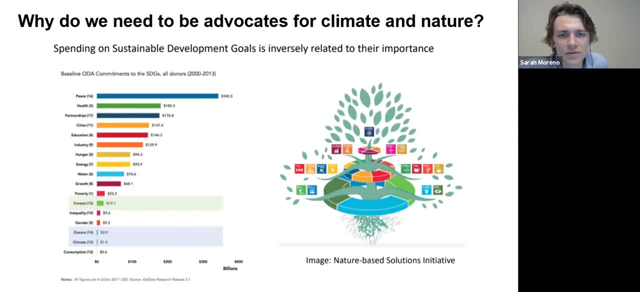 science to factor science and respect the local needs and management. We are going to discuss this a little bit later. So why do we insist so much about nature-based solutions? Basically because there is a huge lack of funding today. So if you look at what they call the wedding cake of the Sustainable Development Goals, 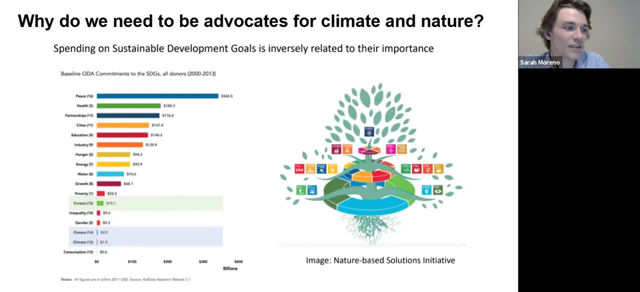 it has different layers. The layer on the right picture, the layer which is underneath It, is the largest one. This one is the base for all the other different needs. So, when it comes to the sustainability of our societies, peace, economies, electricity, 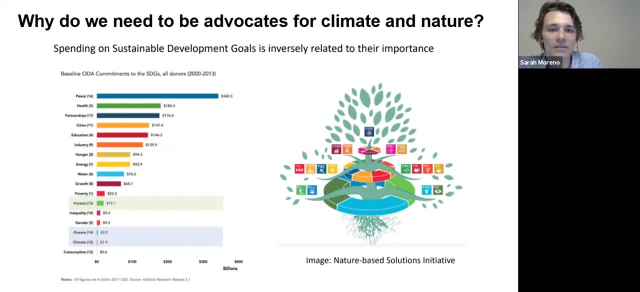 we need to rely on these pillars, We need to make sure that these pillars are well taken care of in order for the rest of the SDGs to be reached. And this pillar? This pillar is basically life on land, ocean, life on earth and climate. 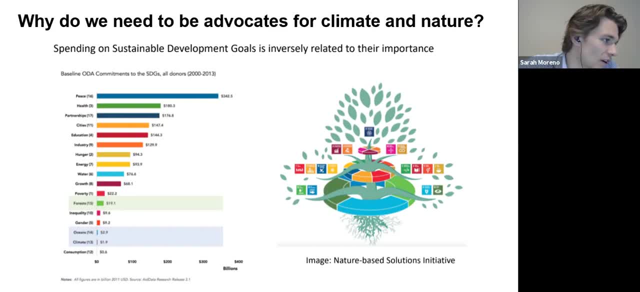 So if you look at the chart on the left, you will see that they are financed the least. So of course, some technological solutions to remedy and to adapt to climate change are more lucrative because you can sell them And you can actually make a profit of it. 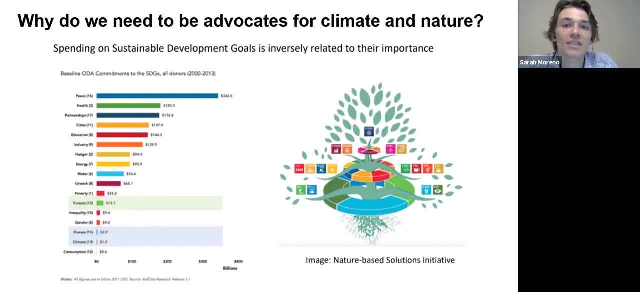 And that's important. That's part of the story. That's a complementary contribution to climate change mitigation and adaptation. But nature-based solutions, especially in the places which are the most vulnerable, are already available: technology, let's say earth technology- that we need actually to. 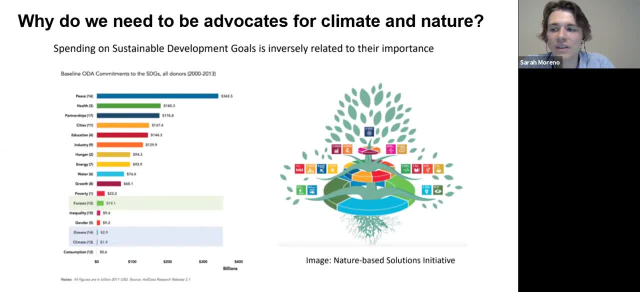 fund And conservation and protection of the natural ecosystem are really important, And I think that's what we need to do. I think that's what we need to do. I think that's what we need to do And that's the social aspect. 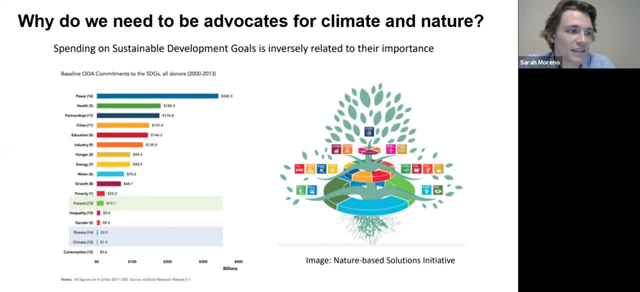 I think that's the recent aspect of finance which is yet to be covered. So we cannot actually forget the nature as a solution And we cannot forget the people, the people who are living and preserving the nature. Climate action cannot do without young people, cannot do without the frontline communities. 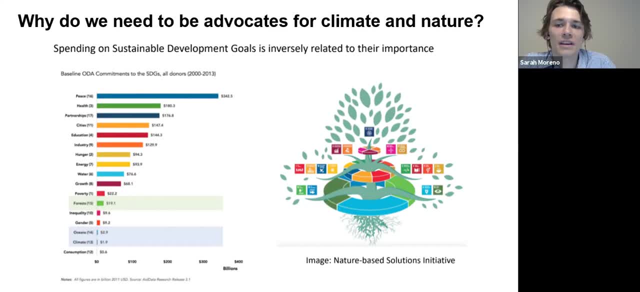 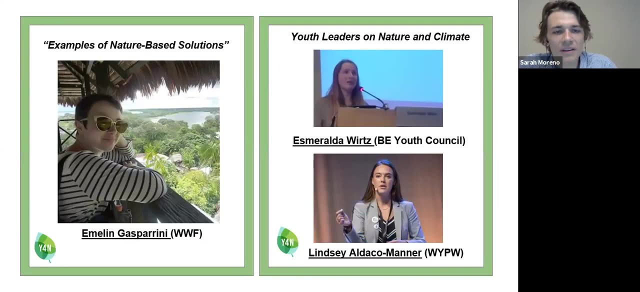 and people Right cannot do without marginalized communities. So what we are willing to do is to empower young people around the world to hold our political leaders to account on both the climate and the ecological crisis. So right now, I will introduce you to our first speaker. 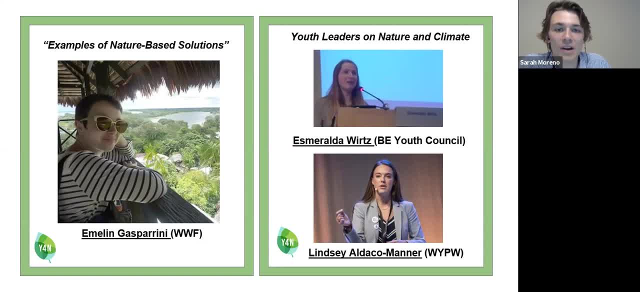 which is from WWF Forest and Climate Hub. I'm very honored to have her here And I would like to introduce Emeline Gasperini. She will tell us a bit about examples of nature-based solutions implementation in the field, With case studies from Guyana and Colombia. 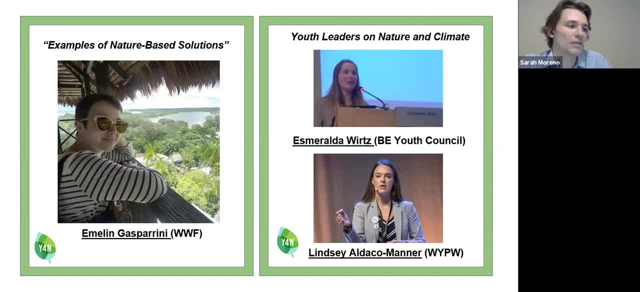 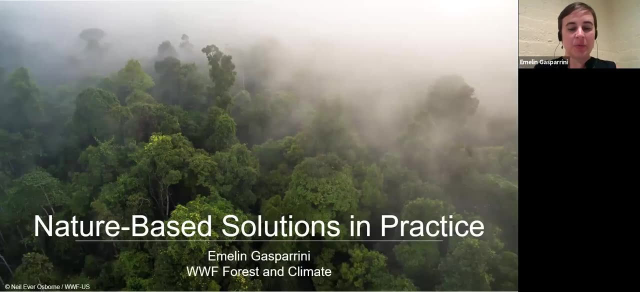 she will speak about WWF work with indigenous community and ecosystem restoration. So now you have the floor. Thank you, Sebastian. So, as he mentioned while he's getting my slides up, my name is Emeline Gasperini and I am a part of WWF's Forest and Climate team. 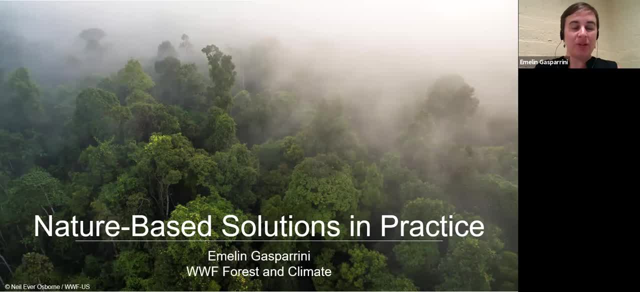 I'm based in DC, but I'm originally from California, which anyone from the US will tell you is something that only Californians say. We insist on our California identity before our American identity. The team I'm on works with our colleagues all around the world. 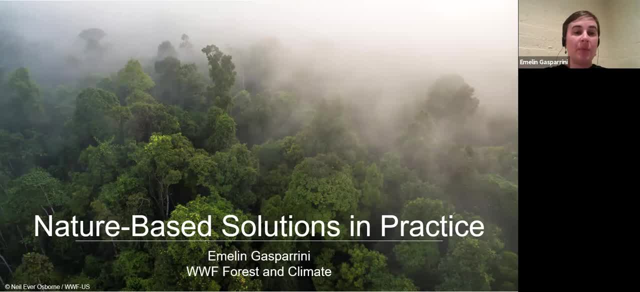 but especially in tropical forest countries, on their forest and climate work as it manifests itself in their individual context, And I really wanna thank Sebastian and Youth for Climate for inviting us to participate and share these examples, And I think that's gonna be a great way. 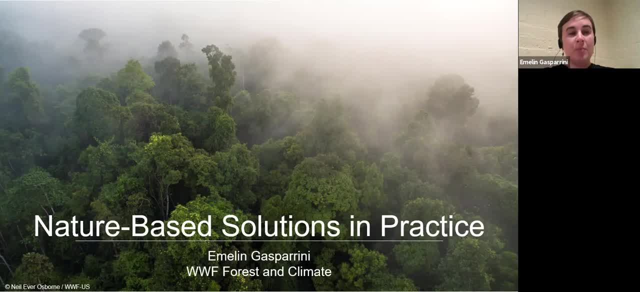 to get the conversation going with all of you And I really liked that you ended your presentation on people and that your definition of nature-based solutions from earlier in the presentation started with the word action, because action is really where people come in And human actions and human choices have obviously led us. 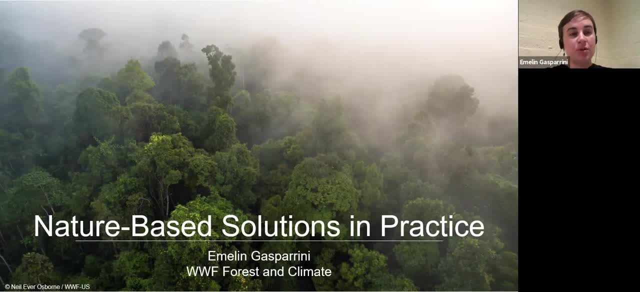 to the climate crisis, and better human actions and choices like those that fall under this nature-based solutions umbrella are really what's needed in the face of the crisis, So I'm gonna share two examples today that are focused on people and how they're pushing nature-based solutions forward. 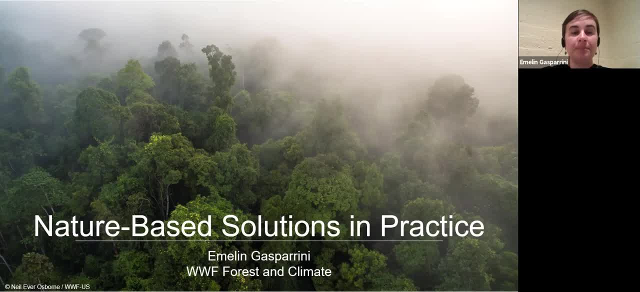 in the places where they live, And I do have publications or stories published about both of these examples. So if anyone wants more information, feel free to drop me an email. I'm very happy to send that around afterwards. We can go to the next slide, please. 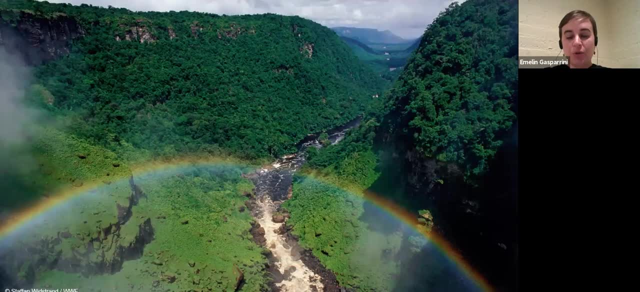 All right. so, starting in Guyana, I would like to take you to the North Rupert and I'm gonna go back to the North Rupert. So this is the North Rupert Nunez in Guyana. It sits in the Guyana Shield. 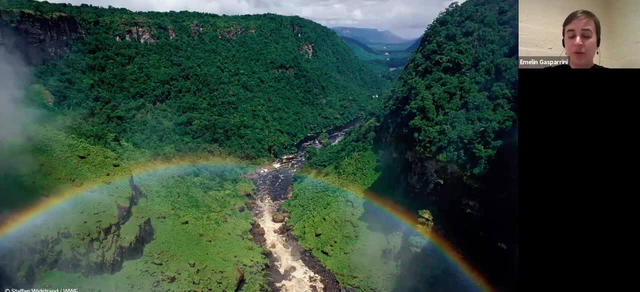 which is the largest remaining block of tropical rainforest in the world. These vast and really biodiverse forests are threatened by mining and timber concessions. a lot of artisanal gold mining happening under the radar and officially, as well as international investment in sort of industrial soy and rice plantations. 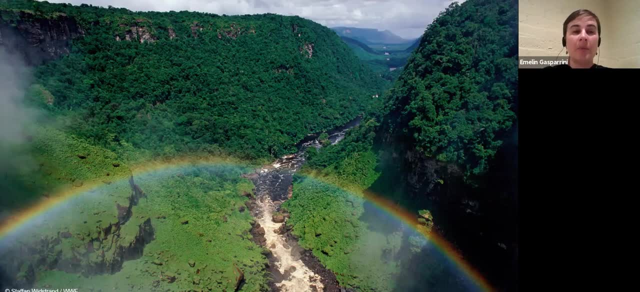 So WWF has been working with indigenous communities here their traditional natural resource monitoring practices they've been doing as part of their culture for millennia in order to have just another layer of information to use so that they can make decisions about that natural resource use. 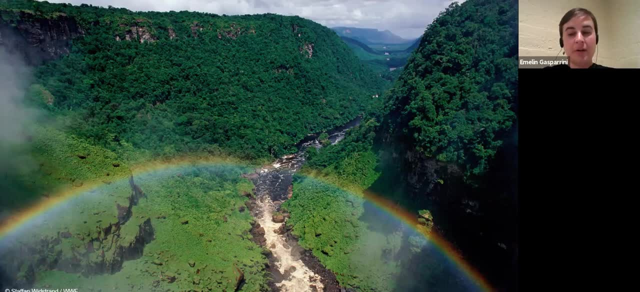 And this tool is called a very wonky name- Monitoring, Reporting and Verification, but it's better known by its acronym MRV, And so MRV. systems are used to collect and analyze data about forest cover, deforestation, forest degradation. 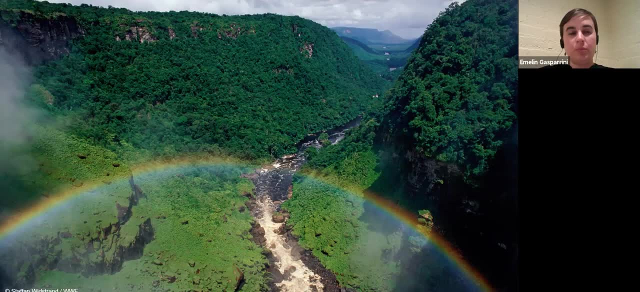 in order to calculate and track emissions from forests- changes in forest cover, all that sort of stuff- And this helps countries determine how much of their emissions are coming from forests and then track any changes in those emissions against their global commitments. that sort of thing. 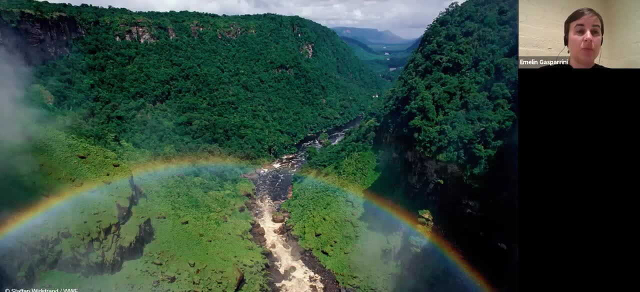 And this is kind of the big picture of what MRV does. but it's actually a really flexible tool. It's why we bring it to communities that want to work with us, because it's really able to be tailored to the context that it's being implemented in. 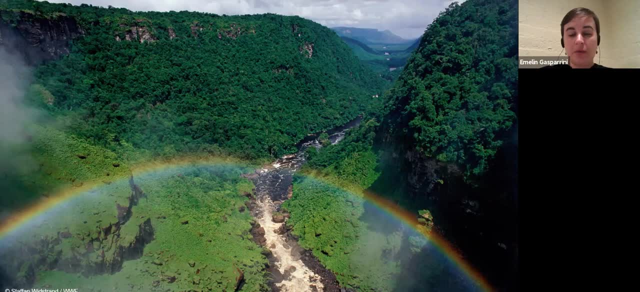 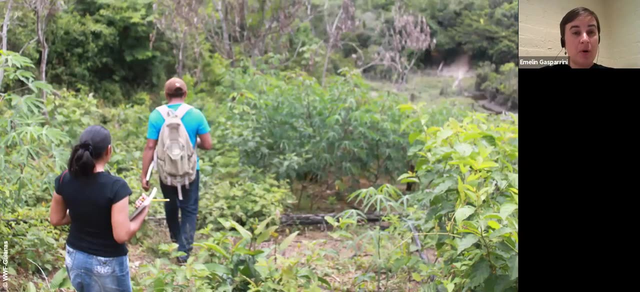 And so this can make it really relevant for those communities that we work with. Next slide, please. And so, with WWF, the communities built MRV systems, called community MRV, and they decided what resources they wanted to track Some communities in addition to their forest targets. 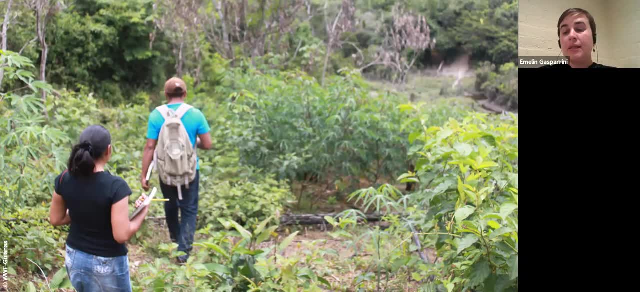 they monitor freshwater fish stocks because that's a dietary staple. some have started to incorporate like public health monitors, especially those that are tied to like changes in freshwater availability, with well depth and all kinds of really detailed, useful, you know, pieces of information that they need and wildlife presence, that sort of thing, and they also select two people to 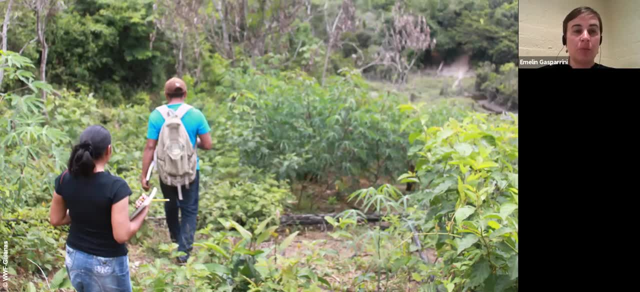 be trained as community monitors and those are the people who are responsible for collecting the data. and a lot of these community monitors are actually young people, you know, in their early 20s, who in this particular part of Guyana also have not that many job opportunities. I spoke with one young man. 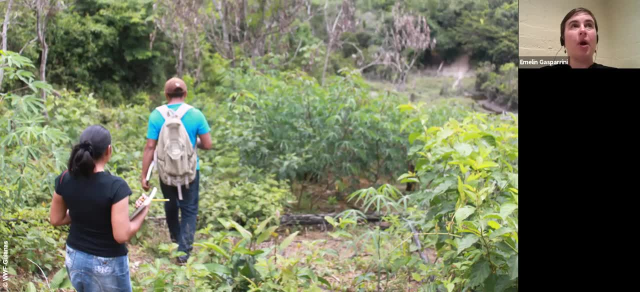 who was really proud to be a community monitor. it brought his village a lot of pride to be able to participate in this program and he said the other jobs available to him really were to go to work in a bauxite mine or to go work on 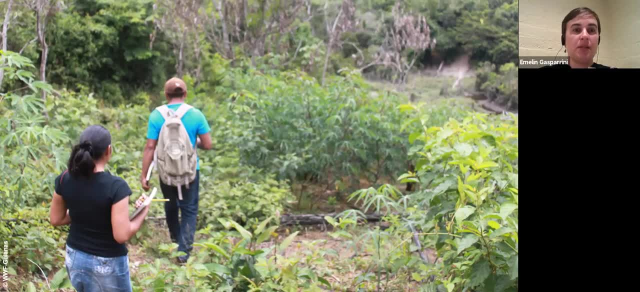 an industrial rice plantation, and so, for him, this was like a much better option for him In terms of being able to support himself and his community. some of these monitors, including this young man, are also trained to analyze this data. so our MRV experts offer technical support, but the communities are the ones who own the 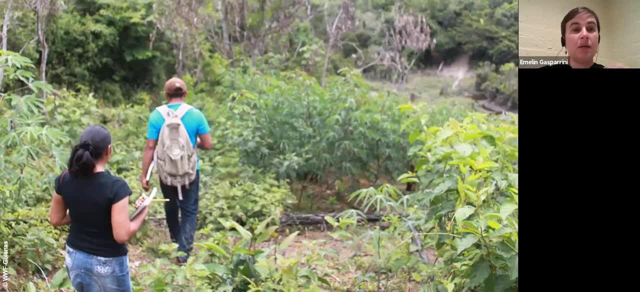 data. they run the analyses, and this is important because a lot of these communities are really remote. internet access is kind of spotty. sometimes electricity access is unreliable as well, and so, by being able to run these analyses by themselves in these dedicated data labs that we've helped them establish, they're not relying on. 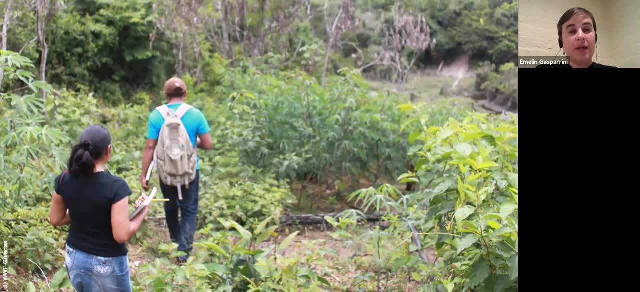 external consultants. they're only relying on us for sort of technical expertise or troubleshooting where they need it, and they own all the data themselves, and especially when working with indigenous communities, that's really important. So they report the forest cover information that they collect to the national government. it's kind of why we can justify having a forest as a 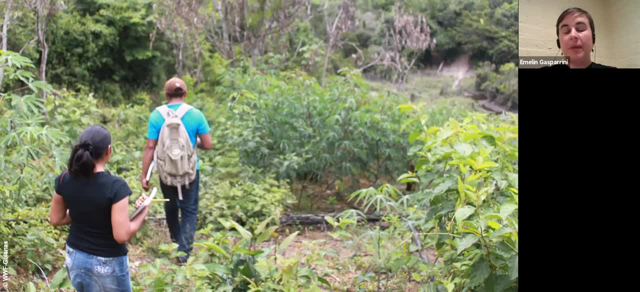 part of the data that we're collecting, and we can't do that without having these MRV systems set up for this purpose. but the data is owned by the communities themselves and they get to decide who they share it with, what they share, and some of the data that they collect they have marked for no sharing whatsoever. so 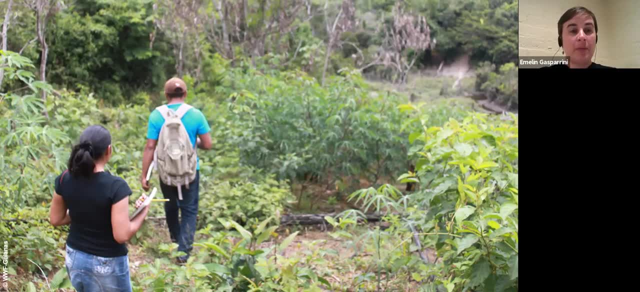 it, nobody can request it and receive that information, and this work is having really tangible impacts on the community's abilities to make those decisions, to monitor their data. One community made changes to their hunting systems in the past year and a half and the data is decreasing at an 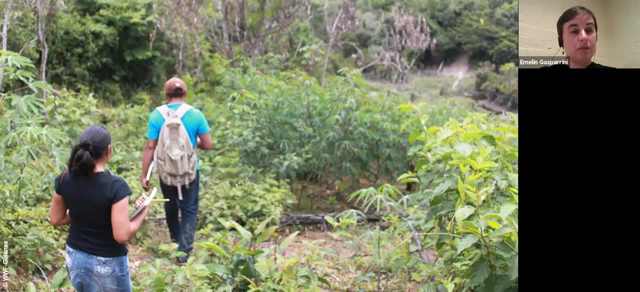 unsustainable rate. Another used this data when choosing new leadership based on the positions that these candidates were offering, and they've all established new rules and regulations based on the information that they've collected in terms of cutting down additional hectares of forests, what kind of natural resource management that they want, community planning and all that. 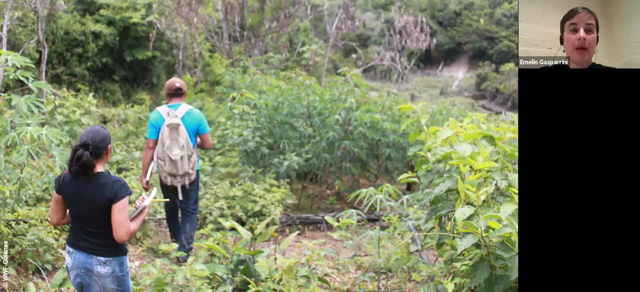 sort of thing, and these communities are using this MRV to manage a million hectares of land and land use. So the BRID and the US Department of Agriculture and Food and Inland Refugee Association have made a much bigger effort for the community to. 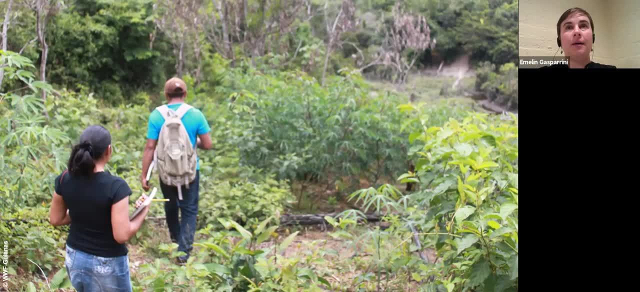 eventually turn this into a place of equal access and meaningful practice for all communities, and the same is true for the community, and it's a lot of work to support people and for the communities and make sure that those communities are being treated with the community-based nutrition that they need to be eating. 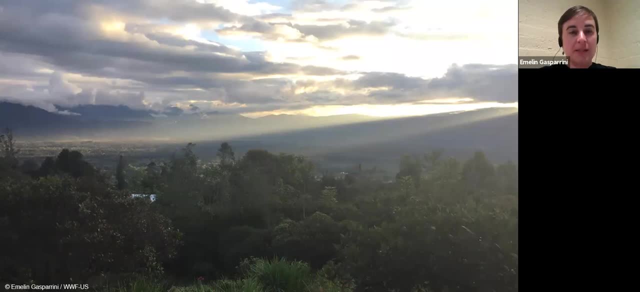 So I'm going to repeat those two points and then I'm going to run through some of the work and some of those work for the community to accomplish in terms of such a significant impact on community development and the community. and in terms of this, I'd like to introduce one person. She's with our National 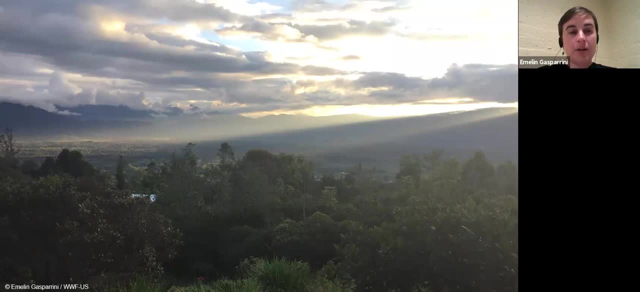 Doña Blanca and she lives in Colombia. She grows granadillo, which is similar to passion fruit, on one hectare of land in this beautiful place, the Sibundoy Valley, but she used to be a dairy farmer, And cattle are a really big driver of deforestation in Colombia and the industry is 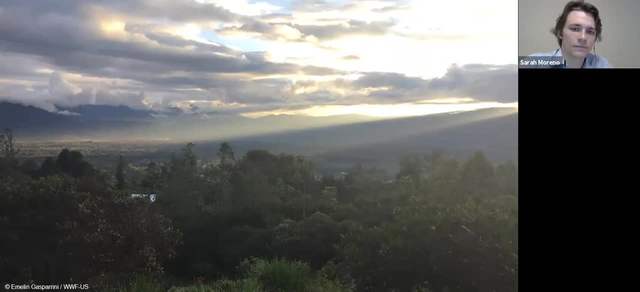 really heavily financed And, especially with the end of the Civil War and the demobilization of park, a lot of the areas that had previously been held by the rebels are, you know, at increased risk of forest loss, Although, for those of you who are paying attention to emissions, changes like 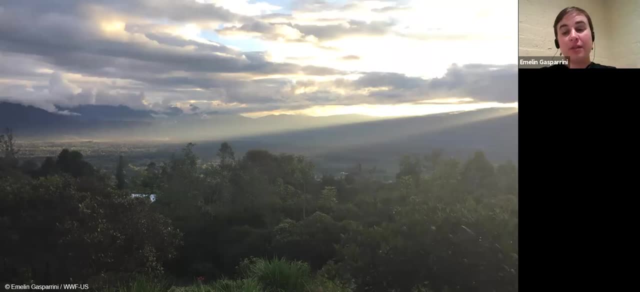 me. Colombia actually reported their first drop in deforestation rates since demobilization three years ago this year, So they're making strides on mitigating those effects as well, But in this part of Colombia, WWF works on the ground with dairy farmers to help them either use more 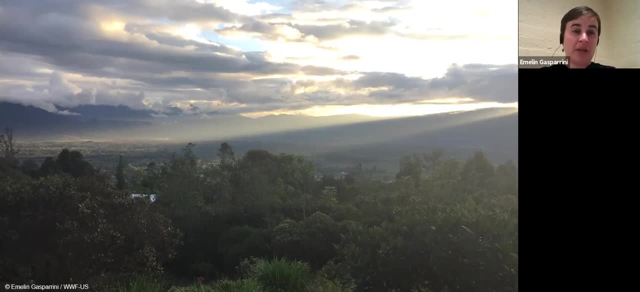 environmentally friendly ways of keeping cows, because dairy is really the basis of their economy and it's all about keeping cows And it's all about keeping cows And it's all about keeping cows And it's also, for a lot of them, really important to their cultural identity, Or, in some cases, 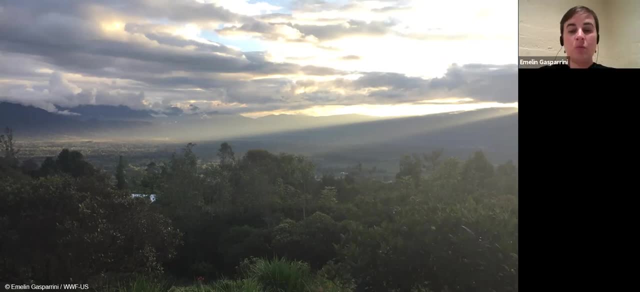 like with Doña Blanca, to move them away from dairy farming to more sustainable land uses and livelihoods. So we worked with Doña Blanca to help her make a plan for her single hectare of land And for American audiences it's kind of hard for us to visualize what a hectare is, since we usually 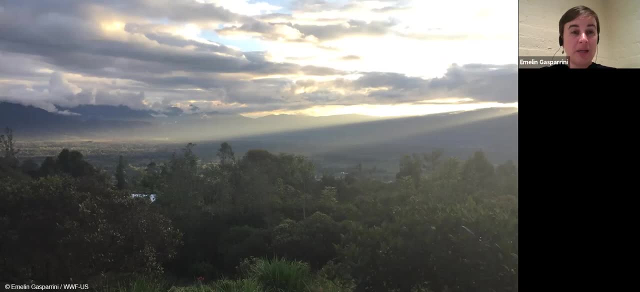 use acres, But if any of you have been on a rugby pitch, it's approximately. it's just slightly more than one hectare. You know it's 100 meters squared, one hectare of land. So it's not a lot of land that Doña Blanca had. 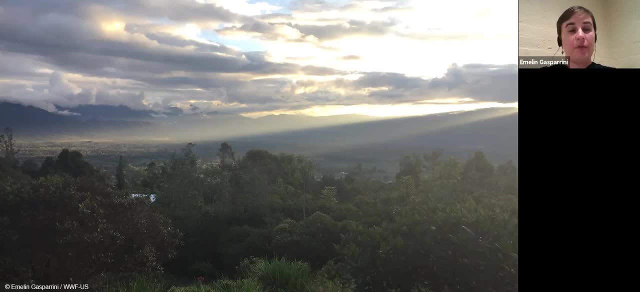 to base her and her family's entire livelihood off of. But we helped her make a plan, And the municipal government, inspired by some of WWF's work, offered a program for reforestation, And so she was able to switch, through this program and, with our support and plan, from dairy to granadilla. 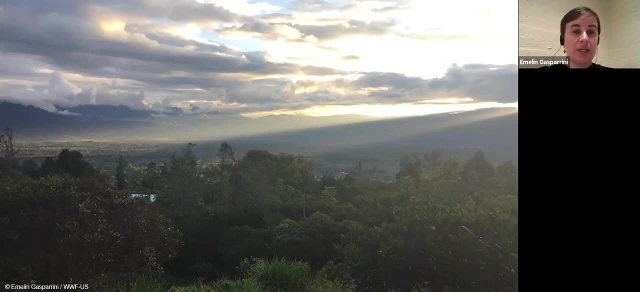 and free up a full half of her land for reforestation without any side effects, And so we were able to sacrifice from her livelihood- And I really want to emphasize- half of one hectare of land that she basically set aside to restore this ecosystem without, you know, needing to take sacrifice in her. 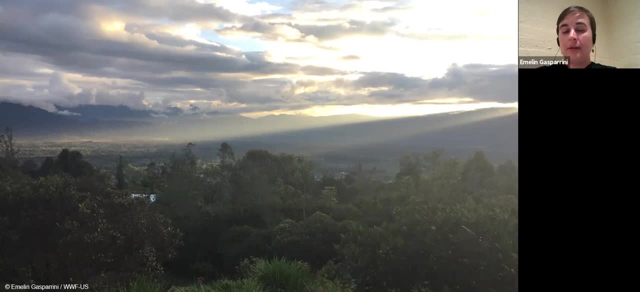 livelihood, which is really, really, for me, inspirational. And so, by planting these trees, Doña Blanca was tapping into the power of forests as a nature-based solution, reducing emissions both from cattle and from land degradation, And also increasing the number of trees in the landscape to absorb the emissions. Next slide, please. 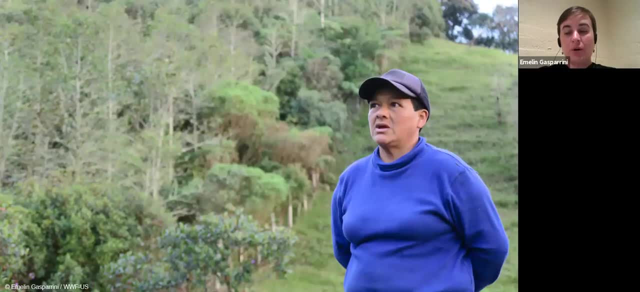 So this is Doña Blanca, And in this picture she's standing next to her forest plot And behind there's a barbed wire fence. you can see sort of along the line of trees there. You go very carefully, climb under that. 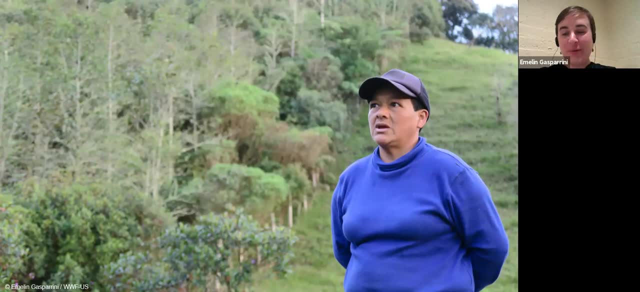 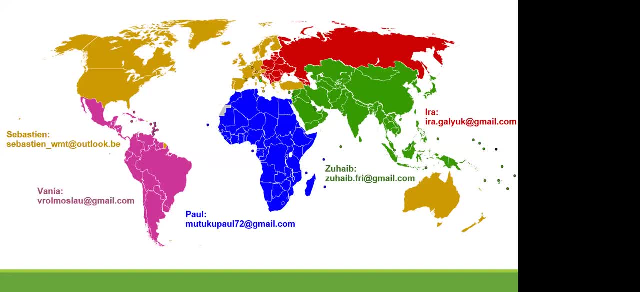 variant answer you: yeah, uh, yeah, i'd be happy to just briefly mention it, but this, this is a platform um and we act as a one of the key partners with it. um, and it's mainly with the global water partnership and the international secretary for water are the the main um platform funders. but 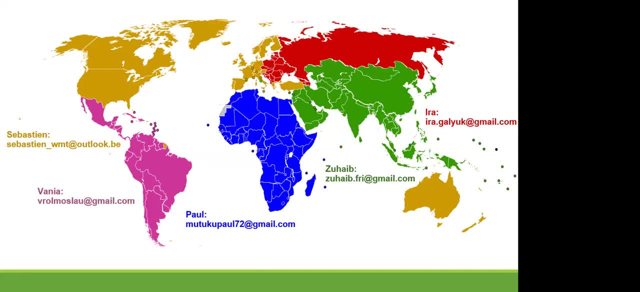 what it does is you submit a project onto the platform, which is, which is basically the website, and there's a process that you go through and on. there is actually some very good tools. this is kind of for everybody in general for submitting, submitting their projects like project development. 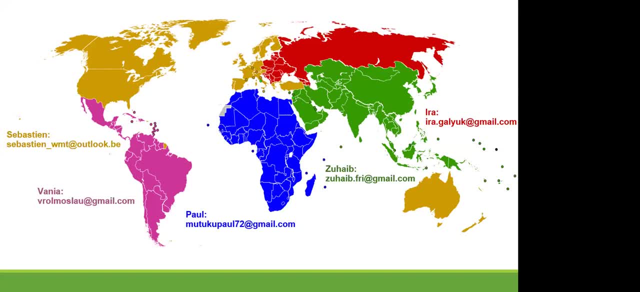 project proposals, that kind of stuff, and then it's reviewed by a committee- um also including youth are on that company, that committee, so it's integrating you throughout the process, and then what they do is they match funders or donors to your project and um specific, i'm not. 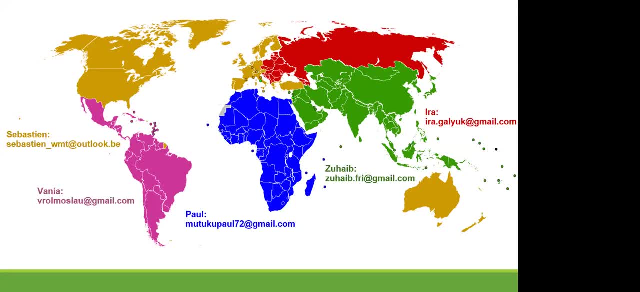 specific um, if they're region based or whatnot, but it's a matching system, if you will, okay, thank you, yeah, thank you very much, of course. okay, thank you so much for asking these very relevant questions and for uh staying until the end with us. uh, i will. i will just repeat. 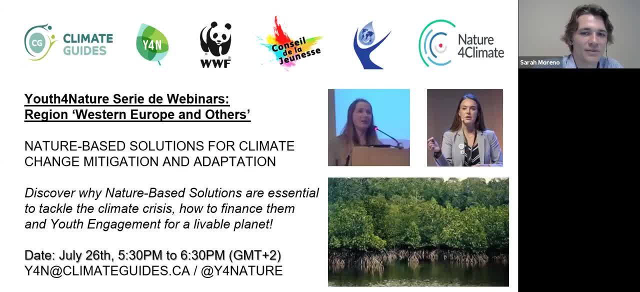 how proud i am to be in contact with all of you and how proud i am of the work that, uh, you're doing. i think this is is very, uh, essential, this fundamental in in our time in history, to make a contribution if we can, and uh, yeah, i i encourage all of you to stay in touch with us and we will. 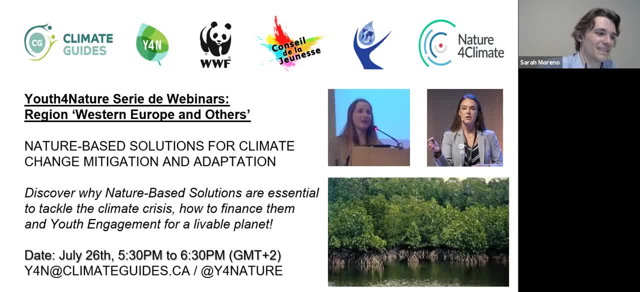 for sure do our part in order to uh contribute, in order to to continue being a relevant actor in that, in that fight. so, um, without uh, i'll just check the chief. yeah, okay, uh. so, without further ado, i will uh put an end to this very pleasant webinar, and i 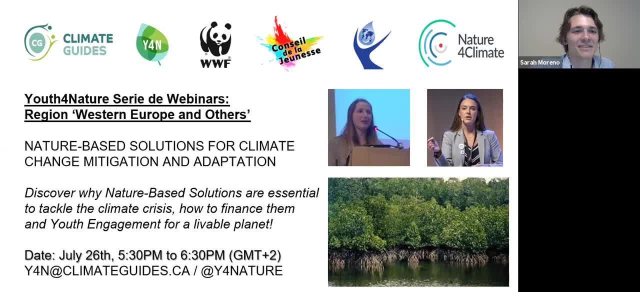 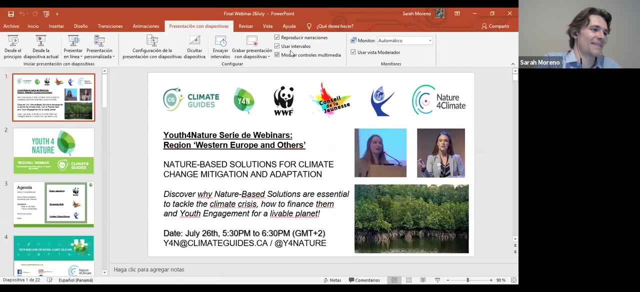 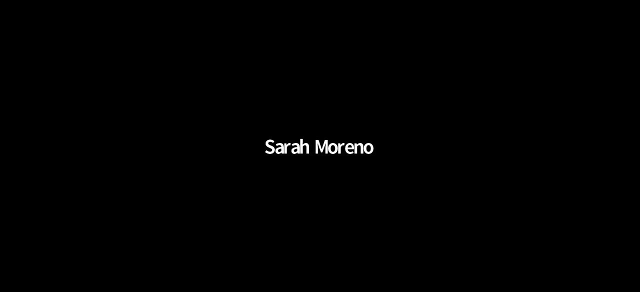 i wish a lovely day to everyone, uh, regardless the time zones which you you are, thank you everyone for making it and thank you everyone for making it so insightful. have a nice day, bye you. Thanks, Lindsay, for putting the link. I see now that you are still sharing some interesting. 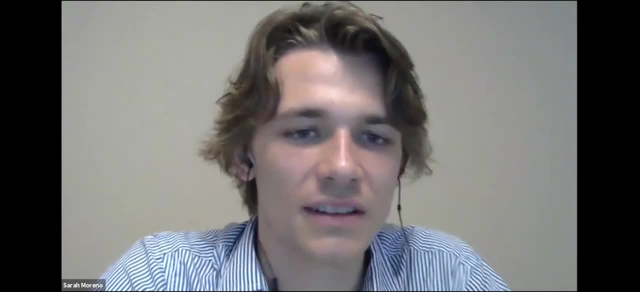 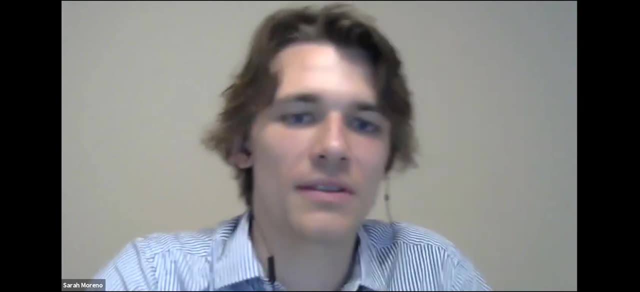 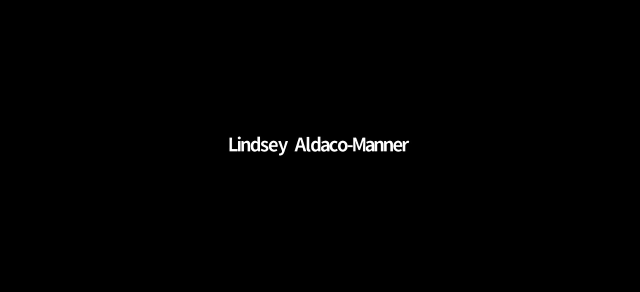 things. Okay, so I will make sure that it's part of the webinar, that you are sharing it and we will try to make them appear. So it's planaearth. Yeah, sorry, just added that one. It's perfect, it's never too late, it's just perfect. 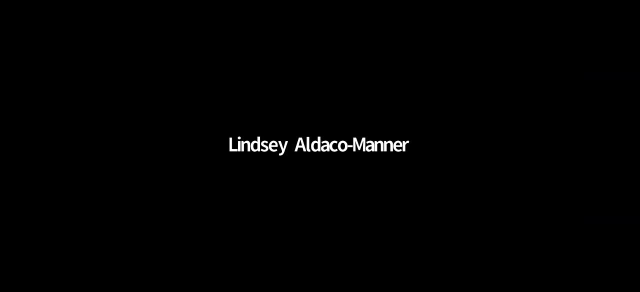 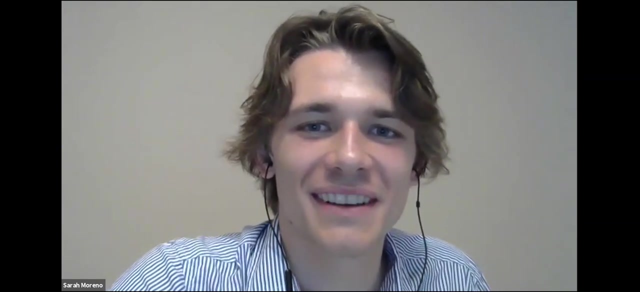 Yeah, this is an excellent platform. I had met the founder at a recent conference and, yeah, want to make sure everybody has a chance to check it out. Everybody has that one. Thanks so much for organizing. It's perfect that at the end it will fit it in terms of time constraint and I'm happy.